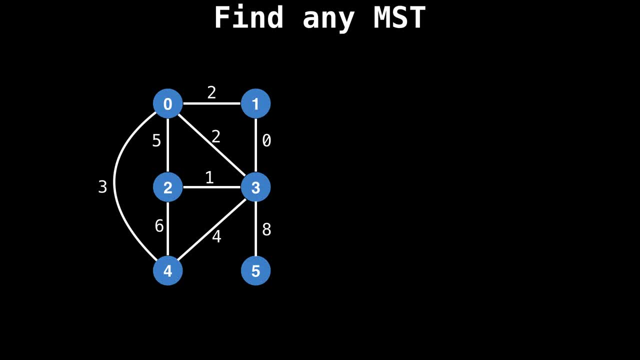 tree you can find. Let's begin with this graph. Take a moment, pause the video and find any minimum spanning tree you can. So one possible minimum spanning tree is the following: with a cost of four: 14. Again, minimum spanning trees are not unique, So there could be another valid minimum. 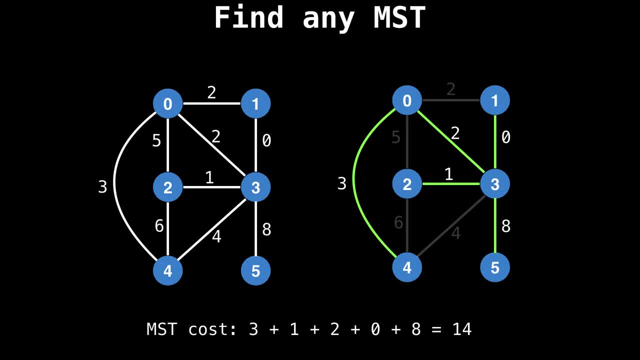 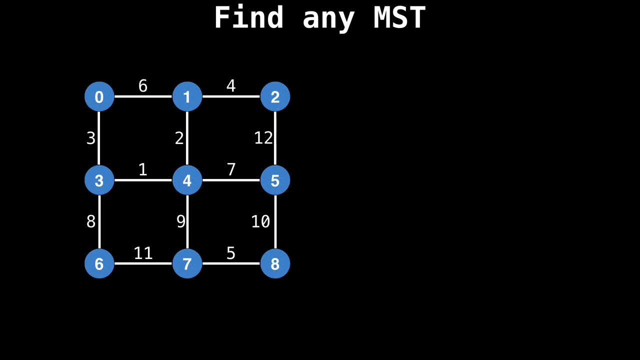 spanning tree here, But they'll all have a cost of 14.. Let's do another one. Can you find a minimum spanning tree here? I'll give you a moment. Here's one possible answer with the minimum spanning tree highlighted in green, with a cost of 39.. All right, one last graph. 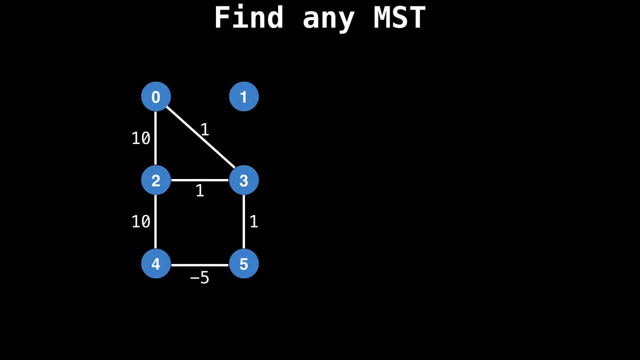 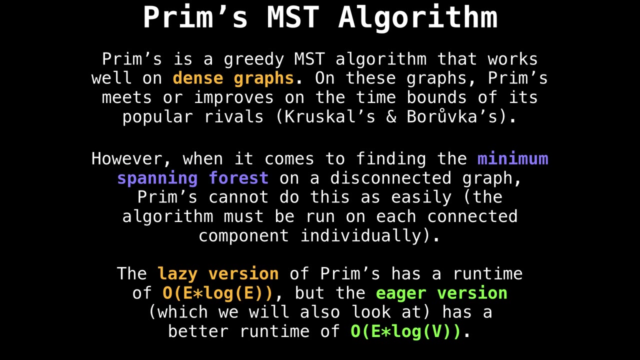 I promise This one is a bit of a trick question because there is no minimum spanning tree. all the nodes must be connected on a single component for a spanning tree to exist. Let's change focus and start talking about prims algorithm. prims is one of my favorite minimum spanning. 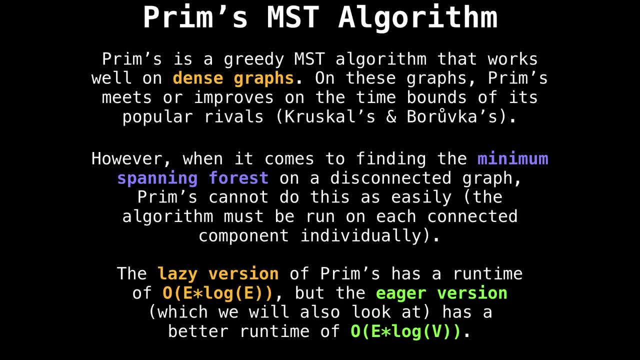 tree algorithms because of how simple and how intuitive it is. By nature, it's a greedy algorithm which always selects the next one. The minimum spanning tree system is basically a simple algorithm that takes the best edge and adds it to the minimum spanning tree, So it works very well on dense graphs, which 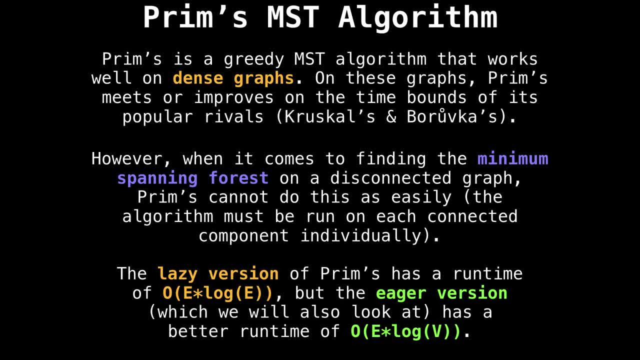 have a lot of edges. However, a few downsides. to prims is that it's not easily parallelizable, or at least not as parallelizable as other well known minimum spanning tree algorithms, And it's slightly harder but not impossible to find the minimum spanning forest of a graph. 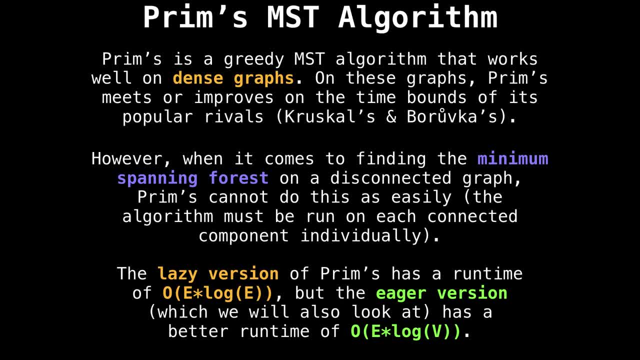 There are two well known versions of prims I want to discuss. The first is the common lazy version, which runs in big O of E log E, And then there's the improved eager version, which runs in big O of E log V but requires a slightly 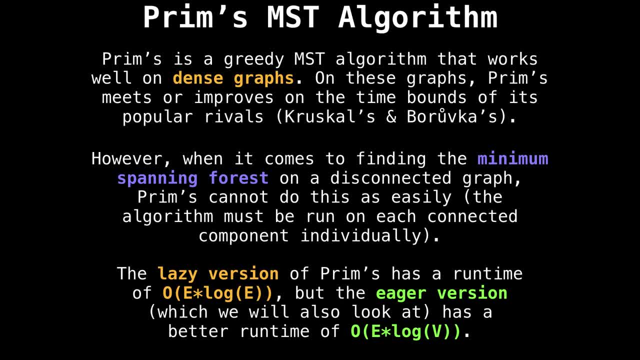 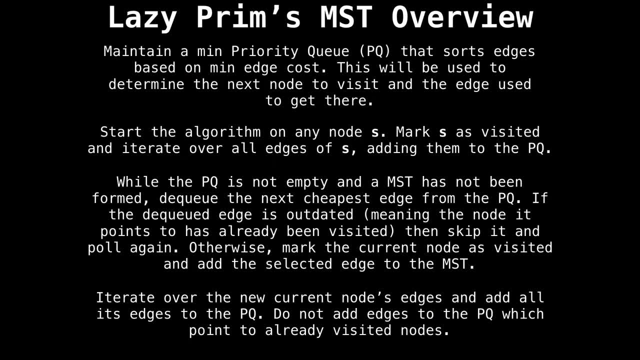 different data structure. We're going to have a look at both, but this video is primarily going to focus on the lazy version. Let's start by looking at the lazy version, Just because it's slightly easier to implement. Here's the general idea: Maintain a priority. 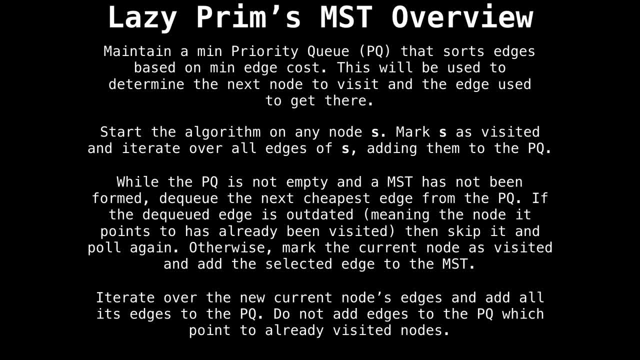 queue that sorts edges based on minimum edge cost. This product queue is used to tell you which node to go to next and what edge would use use to get there. Then the algorithm begins and we start on any starting node s and mark s as visited and iterate over all the edges. 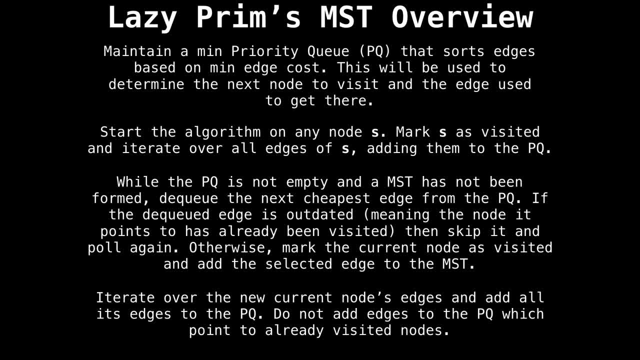 of s and add them to the priority queue. From this point on, while the priority queue is not empty and a minimum spanning tree has not been formed, Dequeue the next best edge from the priority queue If the dequeued edge is not outdated. 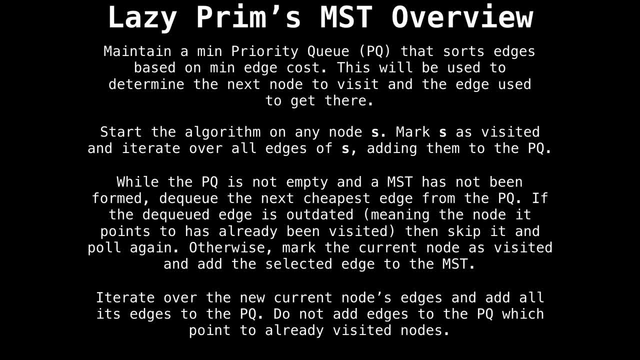 which it could be if we visit the node that edge points to via another path before getting to the edge we just pulled, then we want to mark the current node as visited and add the selected edge to the priority queue. If you selected a stale, outdated edge, then you can. 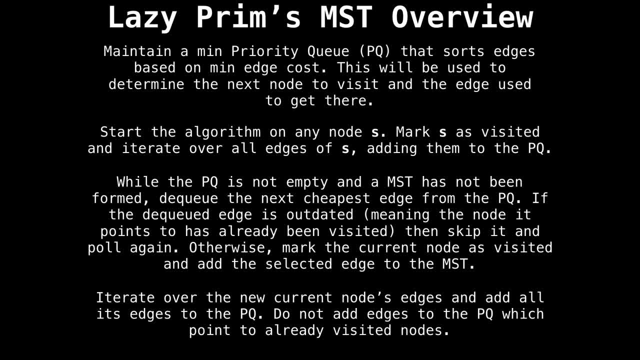 simply pull again, then repeat the process of iterating over the current nodes, edge Edges, adding them to the party queue, And while doing all this, take care not to add edges which already point to visited nodes. This will reduce the number of outdated edges. 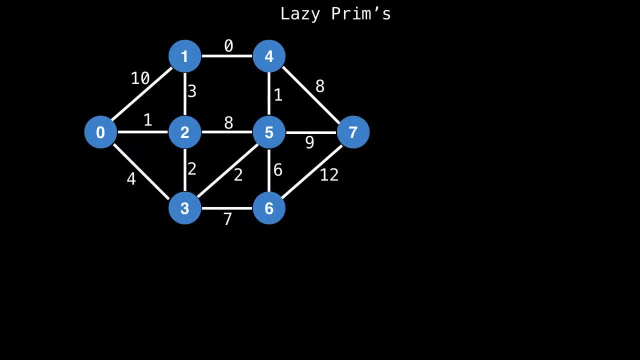 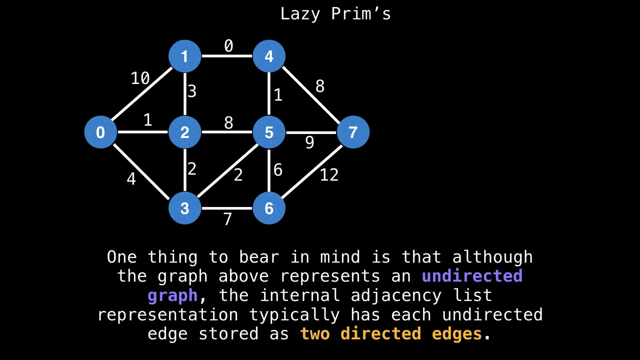 in the priority queue. Let's have a look at an example. Suppose we have this weighted undirected graph and we want to find any minimum spanning tree. An important thing to keep in mind is that, while the graph above represents an undirected graph, our internal 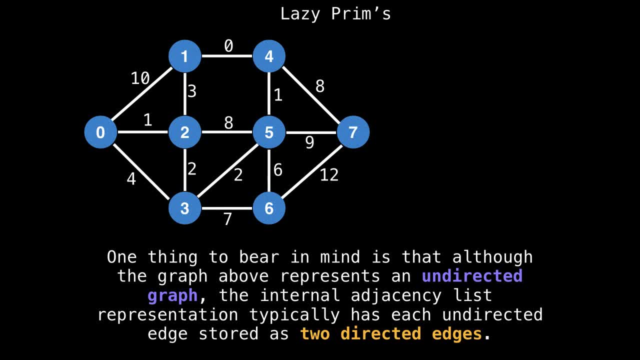 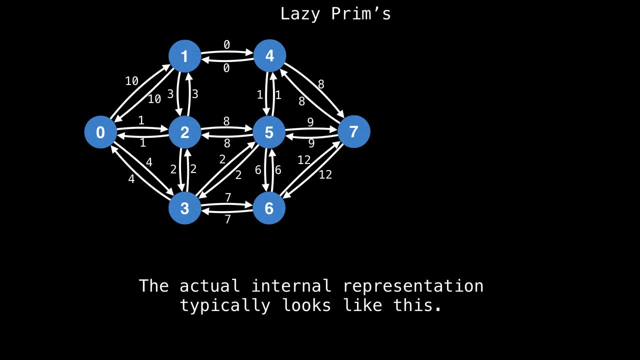 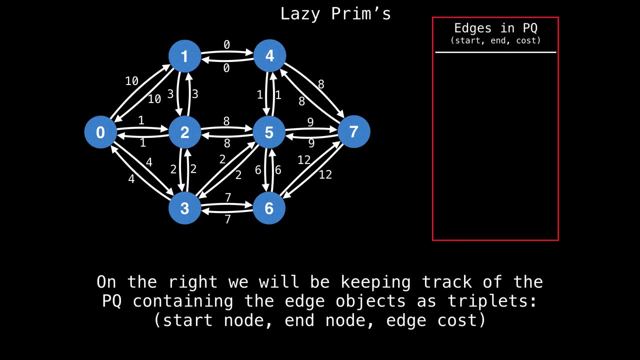 adjacency list representation has each undirected edge stored as two directed edges, So the actual internal representation typically looks something like this, which is a lot easier to work with. Along with the graph, I will also be keeping track of the edges currently in the priority. 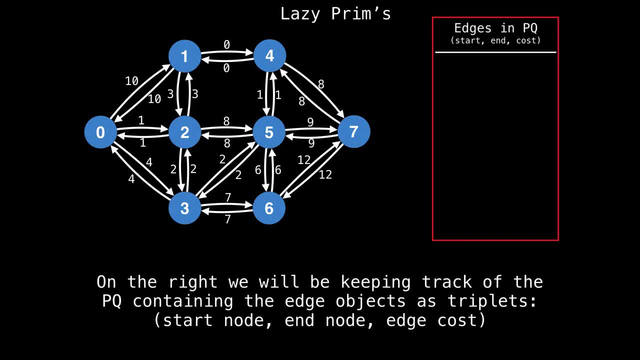 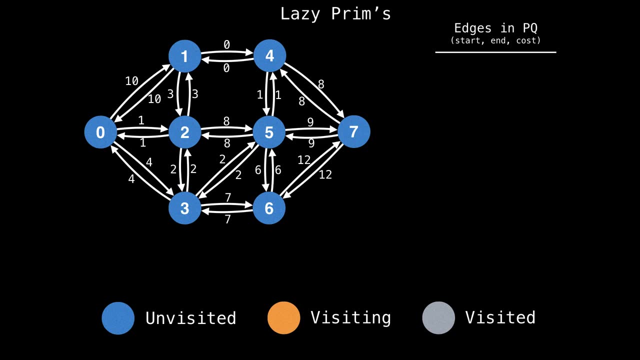 queue. on the right, I will be representing edges as triplets containing the start node of the edge, the end node of the edge and the edge cost. Lastly, I will be coloring nodes as either blue for unvisited, orange for visiting or gray for visited. So let's begin prims on node zero, Iterate over 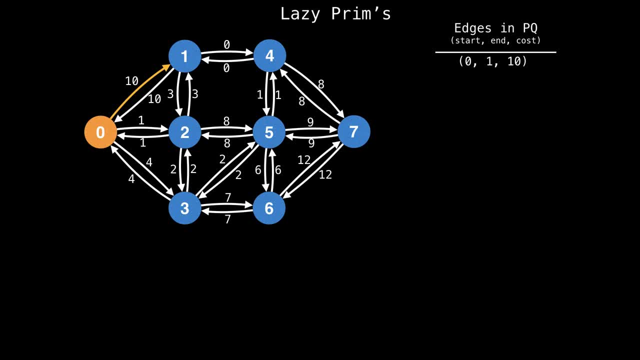 all the outgoing edges and add them to the priority. the first edge we're going to add to the priority queue is the edge from zero to one, with a cost of 10, then the edge from zero to two with a cost of one, And finally the edge from zero to three with a cost of four. Now we look inside our 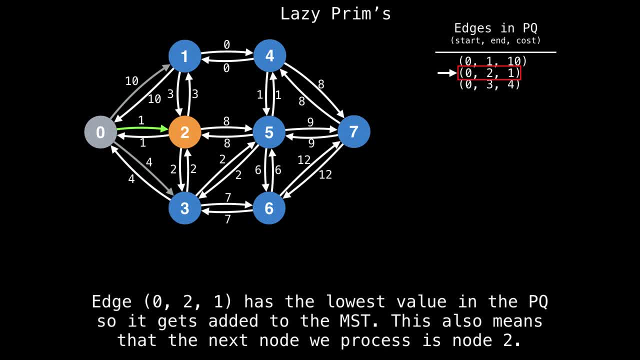 priority queue and we pull the next most promising edge and add it to the minimum spanning tree. the edge from zero to two with a cost of one has the lowest value in the priority queue, So it gets added to the minimum spanning tree. This also means that the next node we process 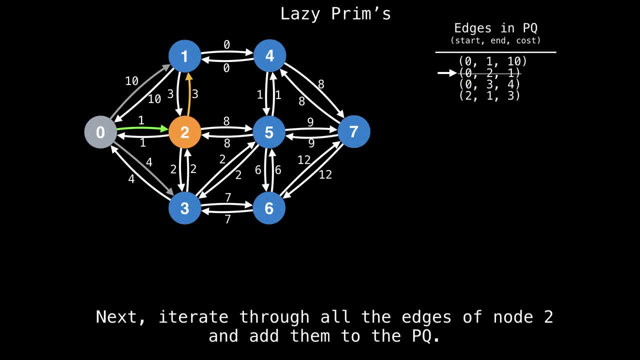 is node two. So next we iterate through all the edges of node two and add them to the priority queue. While entering over the outgoing edges of node two realize that we may encounter edges which point to already visited nodes. we do not want to add these to the priority. 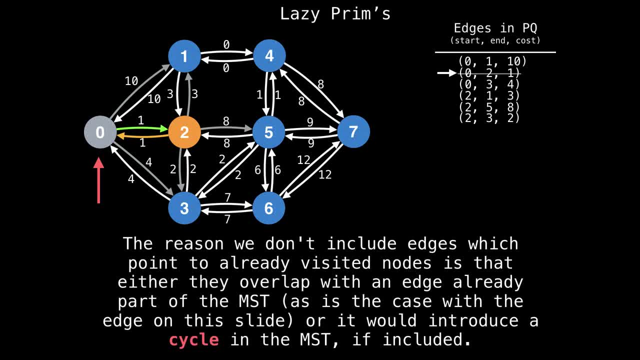 queue because they are of no use. The reason we don't include edges which already point to visited nodes is that either they overlap with an edge already part of the minimum spanning tree, as is the case with the edge on the slide, or they would introduce a cycle in. 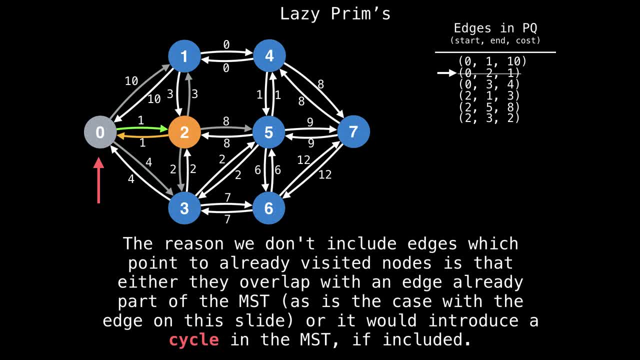 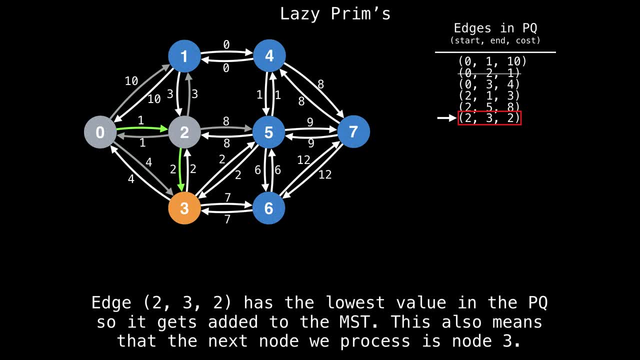 the minimum spanning tree if included, which is forbidden. So the next best edge in the priority queue is the edge from two to three with a cost of two. So it gets added to the minimum spanning tree. This also means that the next node we process is node three. We 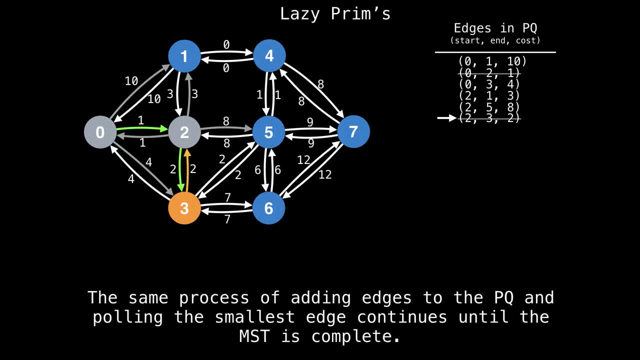 have the same process of adding edges to the priority queue and polling. the smallest edge continues until the minimum spanning tree is complete. I'll let the animation play until something interesting happens. Now let's go to the next stage. Let's go to the next stage. 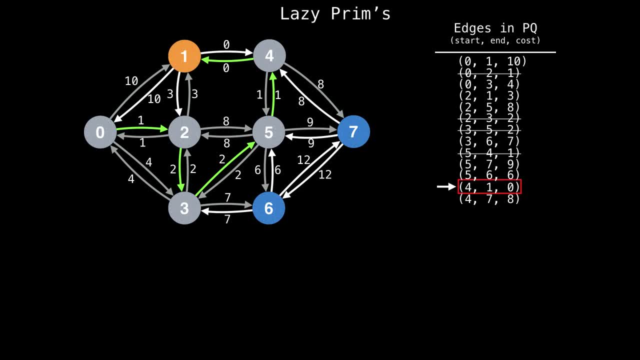 So let's create another value. So let's create another value, Alright. notice that the next best edge we pull from the priority queue is an edge which already points to a visited node, node one. This means that the edge is outdated and stale. 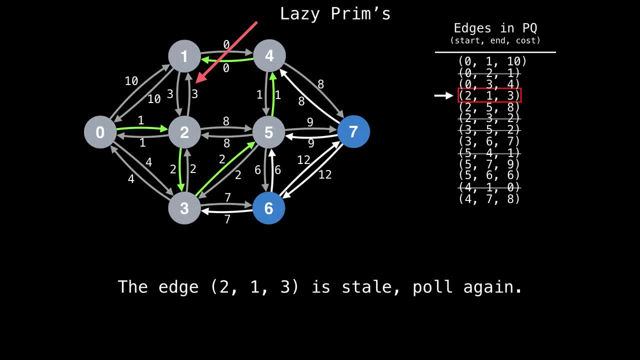 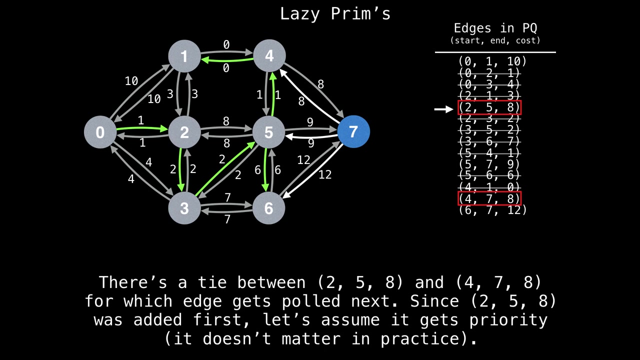 because we found a cheaper path to node one, So we can safely ignore this edge and pull again. The next edge is also stale, So let's keep pulling. So what happens when we have two edges with the same cost in the priority queue? Which one gets pulled first And what? 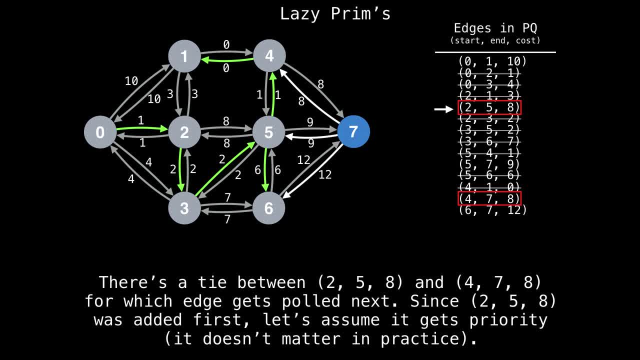 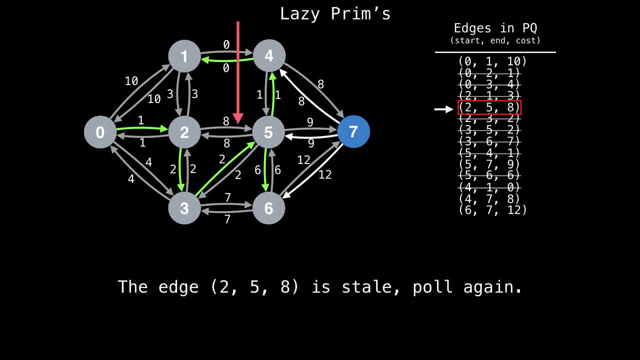 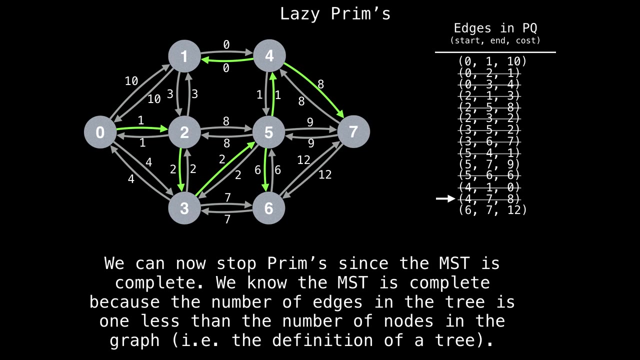 in practice this doesn't matter. So we can assume that edge 258 gets pulled first because it was added first. We can now stop prims because the minimum spanning tree is complete. We know the minimum spanning tree is complete because the number of edges in the tree is. 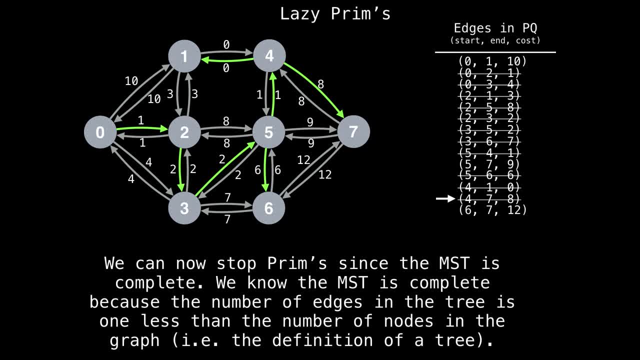 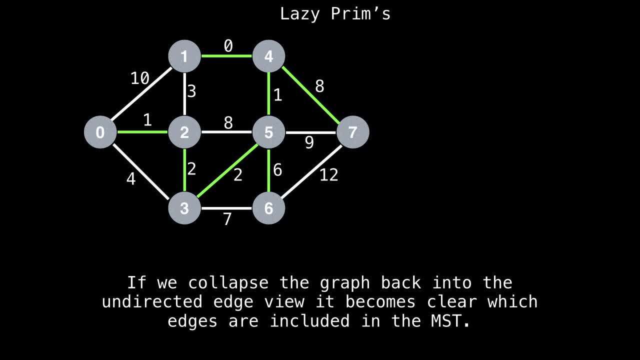 one less than one, Then the number of nodes in the graph. This is precisely the definition of a tree. If we collapse the graph back into the undirected edge view, it becomes clear which edges are included in the minimum spanning tree. To find the cost of the minimum spanning tree: 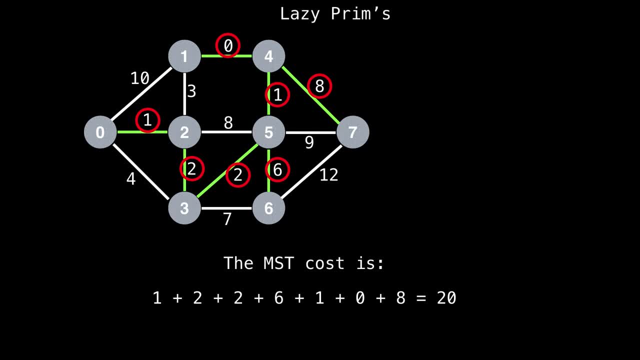 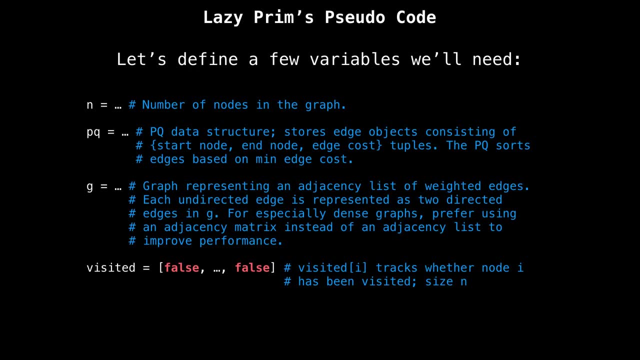 is simply sum up the cost of all the edges which were selected to be part of the minimum spanning tree, And this totals to 20.. Great, we now understand the gist of the lazy implementation of prims. Let's have a look at some pseudocode. Let me first define a. 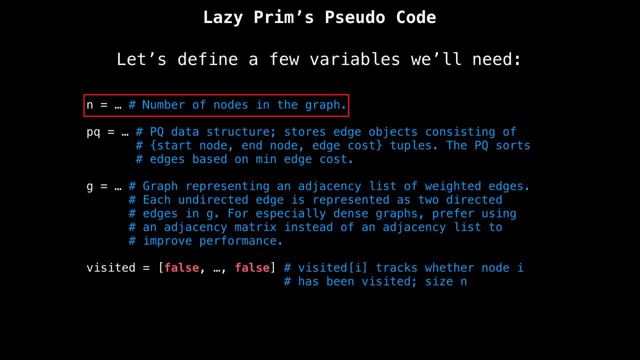 few variables that we will need. First is n the number of nodes in the graph. The variable PQ represents the priority queue data structure. It stores the edge objects based on minimum edge cost. Again, each edge object consists of a start node and end node and an edge cost. 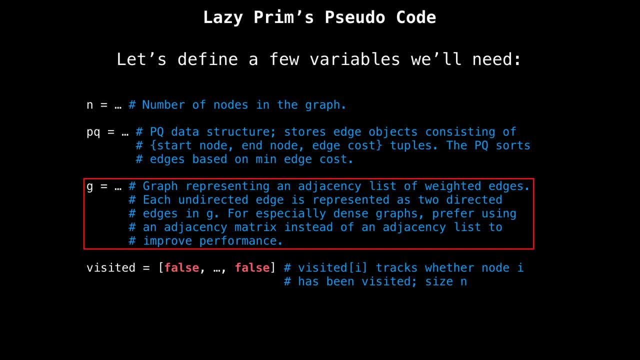 Next is G, which represents the graph we're working with. G represents an adjacency list of weighted edges. In G, every undirected edge is represented as two directed edges. As a side note, if your graph is extremely dense, meaning it has numerous edges, you 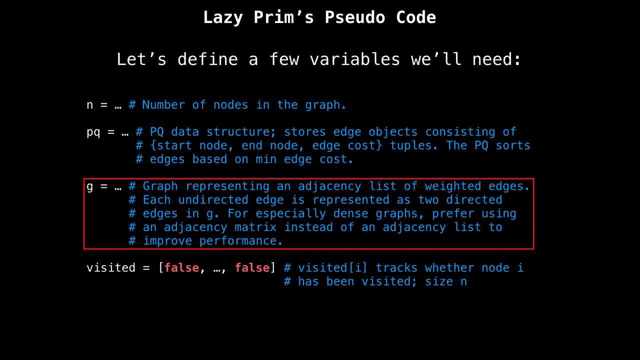 should probably prefer using an adjacency matrix instead of an adjacency list for efficiency and space gains. And lastly, a visited Boolean array of size n which keeps track of whether node i has been visited or not. So on this slide is the whole algorithm for the lazy. 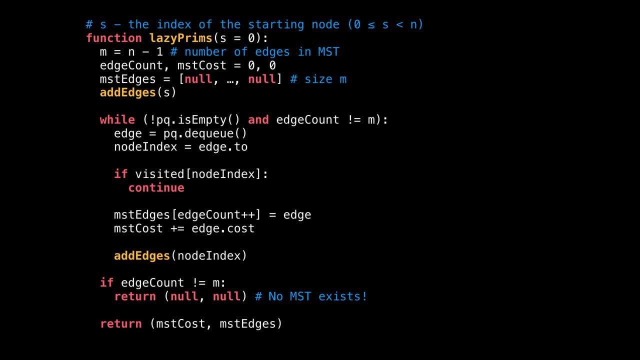 implementation of prims. Let's go over it one step at a time. The function takes one argument, s, which is the start node index, And by default s is set to node s And we set it to node zero. Then I define a few more variables that we'll need just inside. 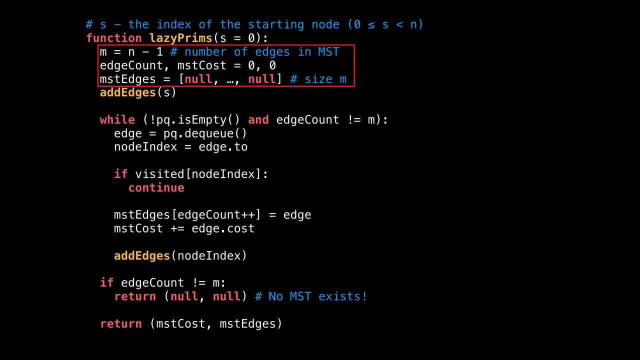 this function. M is a constant representing the number of expected edges in the minimum spanning tree. edge count is the number of edges we currently have included in the minimum spanning tree. This variable is to make sure that the tree spans the whole graph, MST. 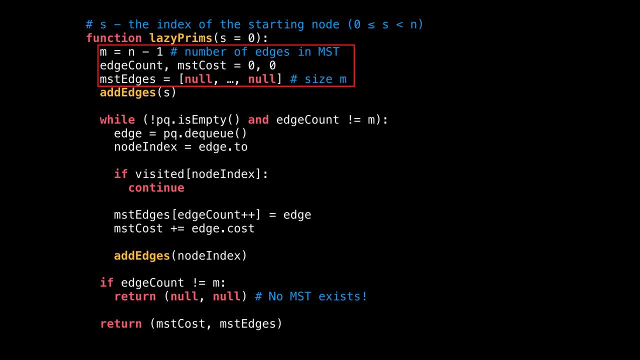 cost tracks the total cost of the minimum spanning tree And finally, MST edges are an array which holds edges which we have included in the minimum spanning tree. The first actual bit of logic we do is add all the outgoing edges from s to the priority queue with the. 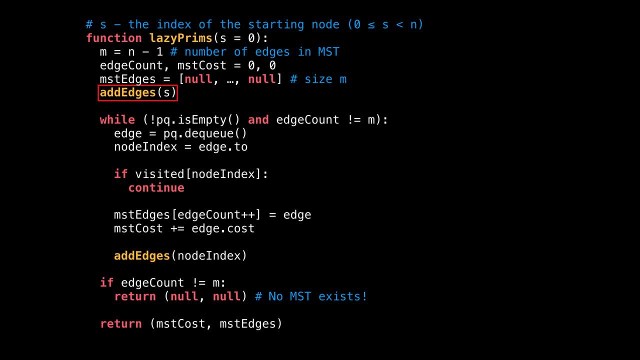 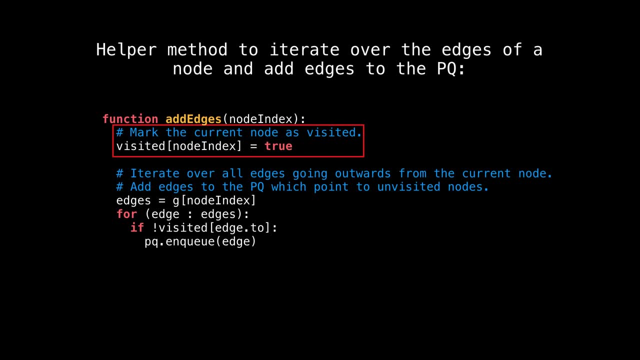 add edges method. So let's look at this method and see what's going on in there. All right, here we are at the add edges function. The first thing I do is mark the current node as visited. Next I iterate through all the 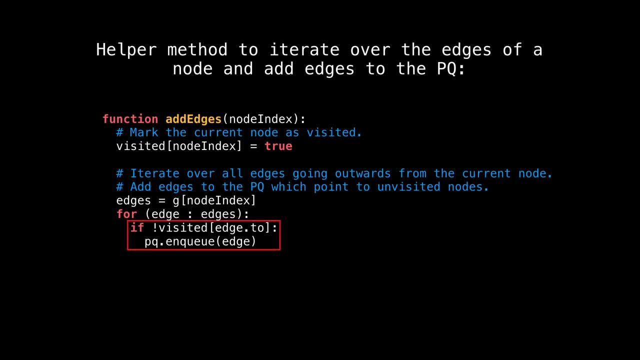 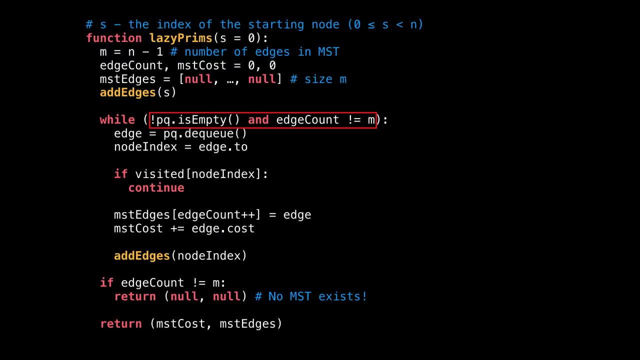 outgoing edges of the current node And if the destination node is unvisited, add the edge to the priority queue. So that's all this method does, is it goes through all the edges of a node and adds them to the priority queue if appropriate. Once we've added the